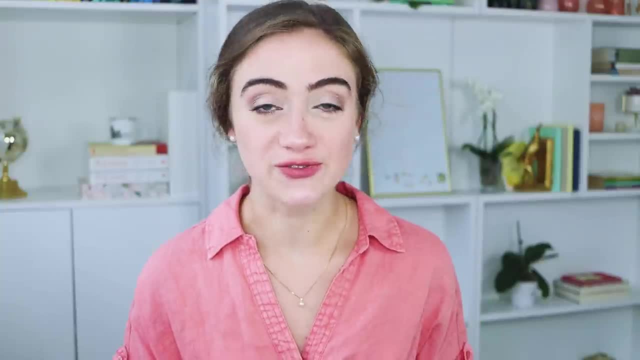 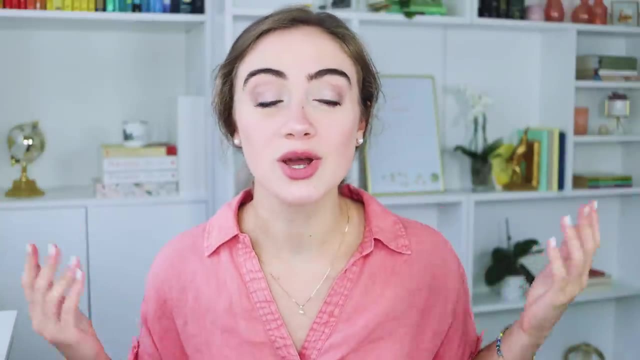 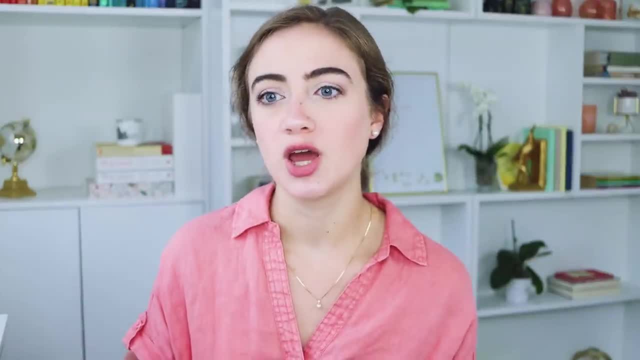 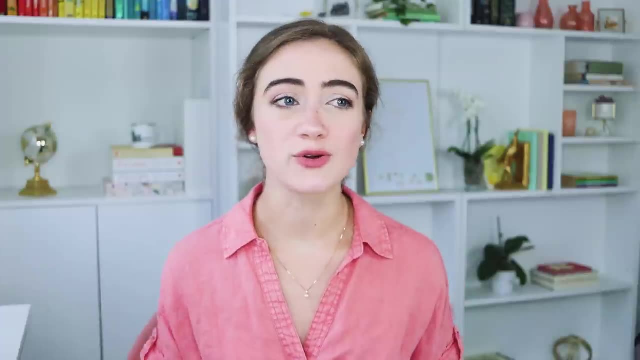 Well then, that I don't have any prior emotional connection to, so if I don't care about it, how will my reader care about it? If writing prompts don't work for you, but you need to write something. you want to write something. you want ideas and inspiration in this video. 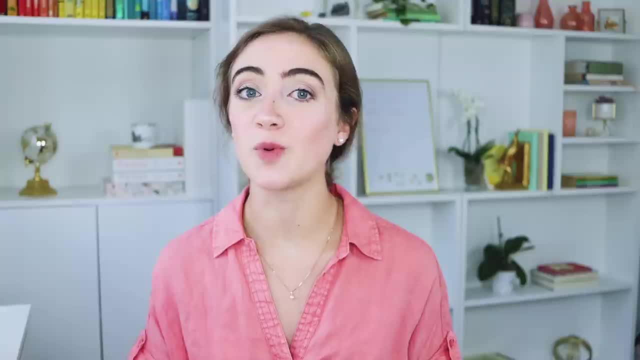 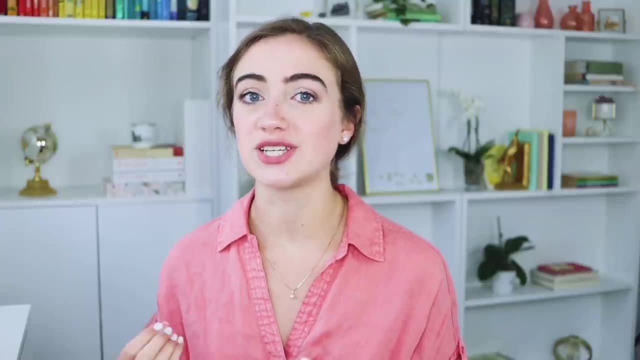 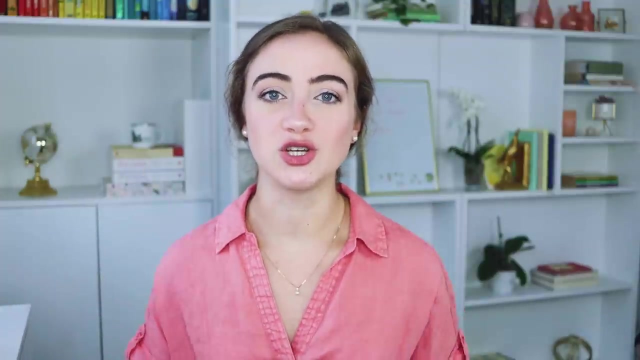 I'm going to share with you a great method for coming up with story ideas when you have no ideas and no inspiration: by drawing inspiration from stories that get you really excited, Creating a story that is unique and memorable and matters to you. Roll that intro and let's get started. 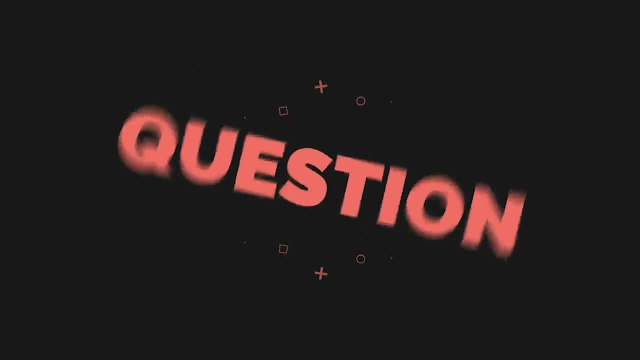 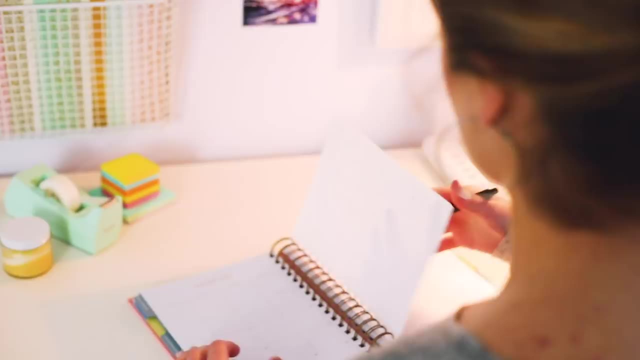 Why does your story matter? Good question. What if I told you that there's a science behind every great story? I don't just teach you how to write, I teach you how to change the world with your story and make your author dreams come true. 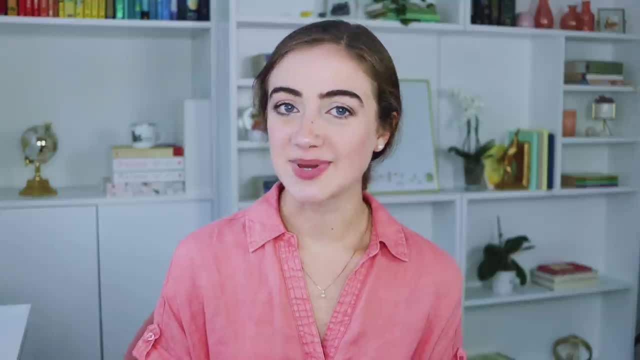 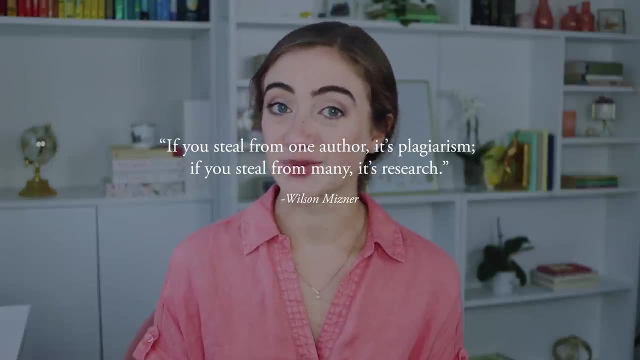 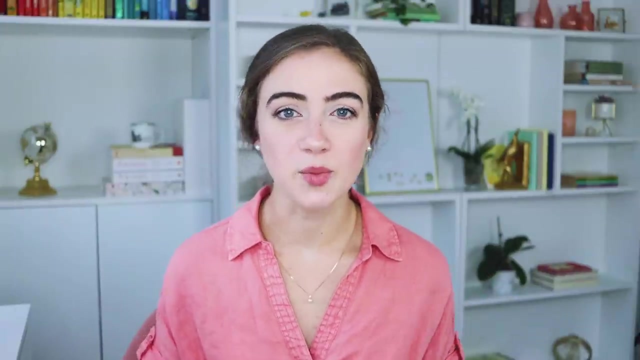 Wilson Misner once said: if you steal from one author, it's plagiarism, If you steal from many, it's research. All ideas are stolen, even ones that seem original. Coming up with a story idea that's all your own really just consists of gathering bits. 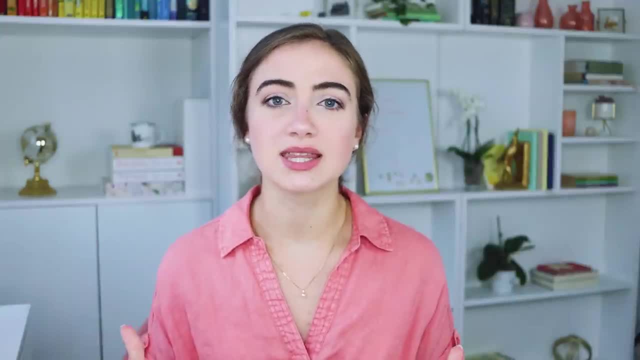 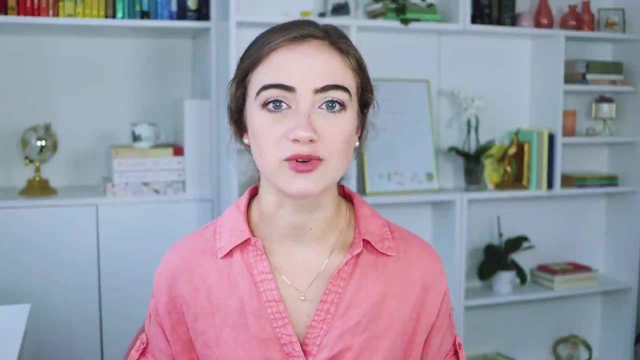 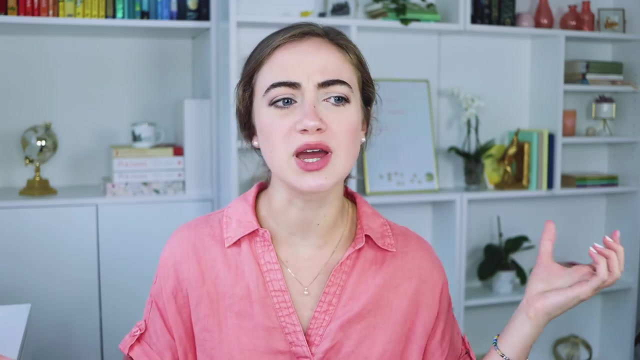 and pieces of other stories and remixing them into your own arrangement to create your own story. It's kind of like creating your own recipe. You don't just start throwing things together and hope for the best. You take inspiration from other recipes, You combine things, You take parts and 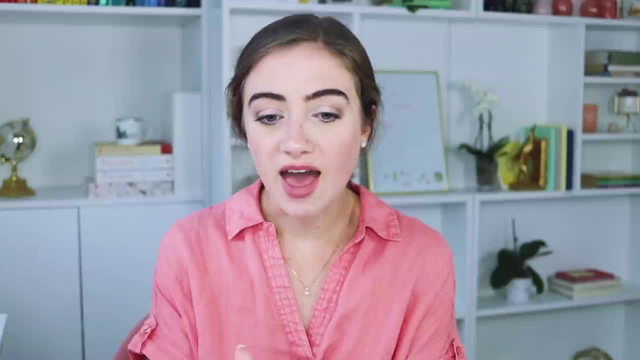 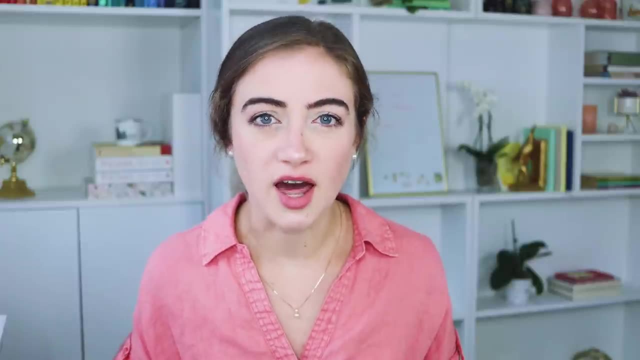 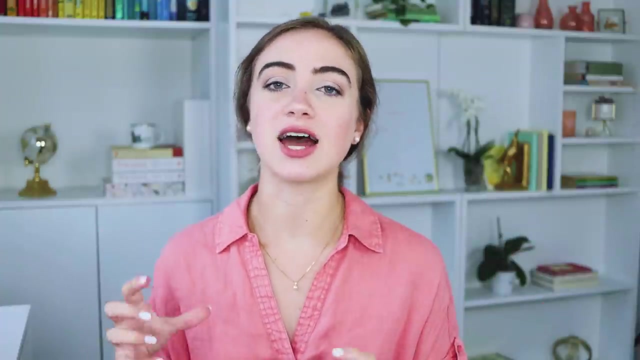 pieces, mix them together, You create your own arrangement, and that now becomes the unique thing that you created. but you didn't start from nothing. So this exercise that I'm about to show you is not so much about stealing. Don't think of it as stealing. Think of it as drawing inspiration. 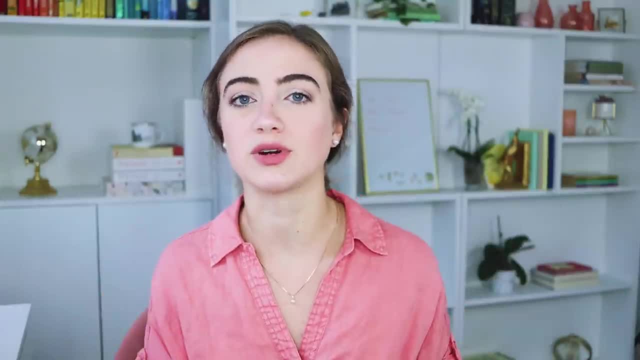 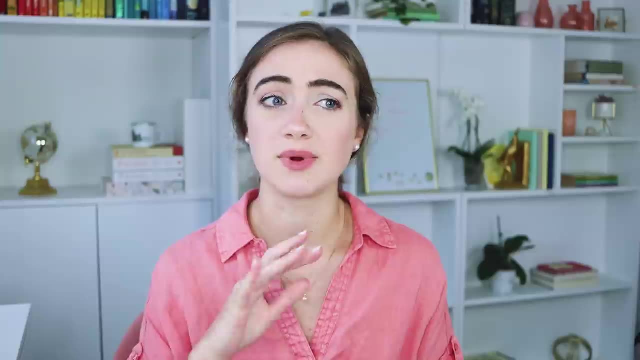 from other sources. There are really only a few stories, And they all just get retold in different ways. Every great writer draws inspiration from other stories, And in a minute I'm going to show you some examples of this, But for now I want to 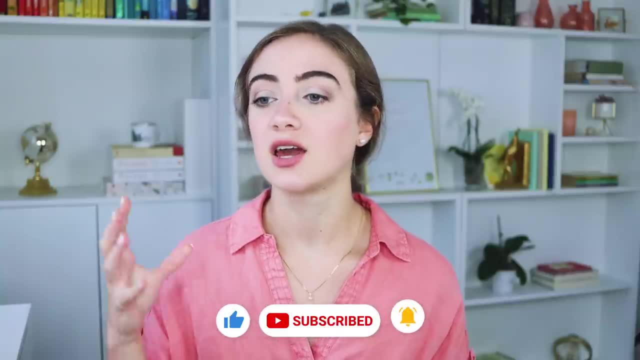 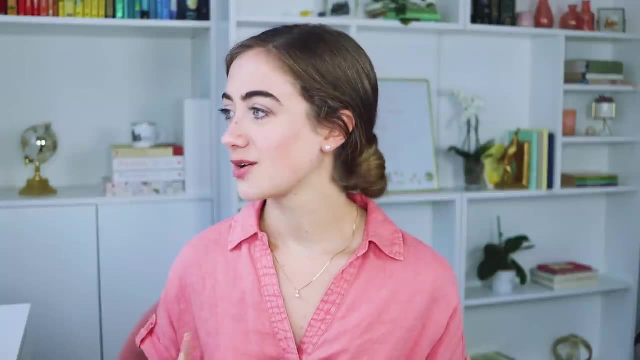 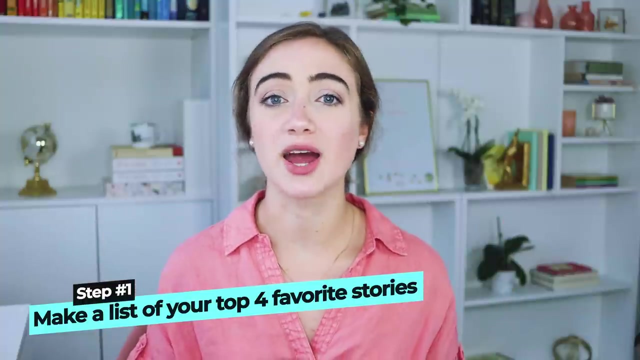 show you the method for coming up with unique ideas using stories that matter to you, so that you can write a story that matters too, Rhyme. Okay, First step is to make a list of the top four favorite stories that you've read or watched recently. that got you really. 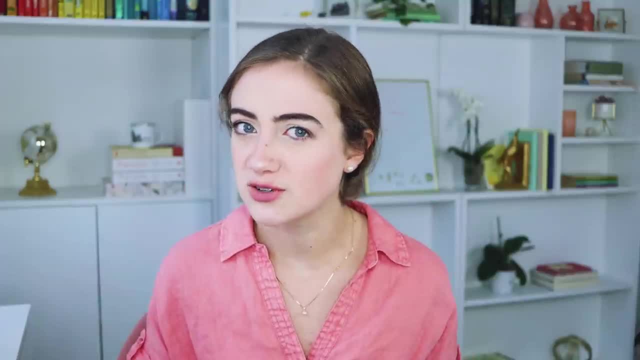 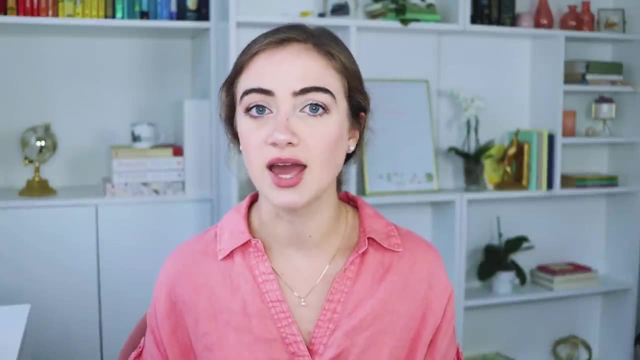 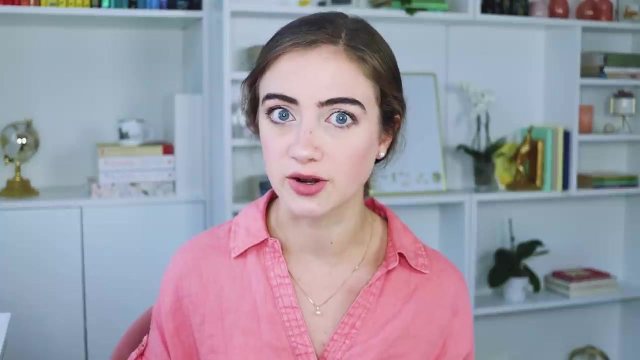 excited and creatively inspired. It doesn't have to be just four. You can make a giant master list of these- In fact, I recommend doing that- but you have to come up with at least four. Okay, And they can be old favorites, but try to choose ones that still get you excited and creatively inspired. 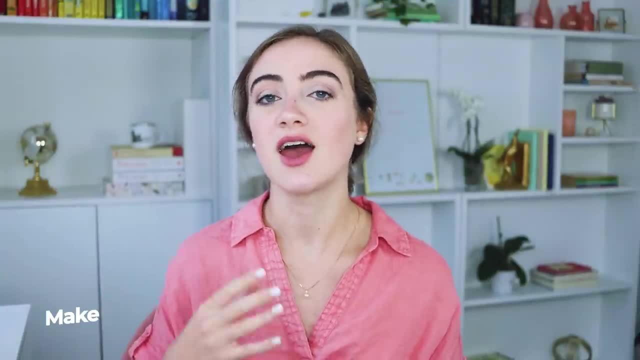 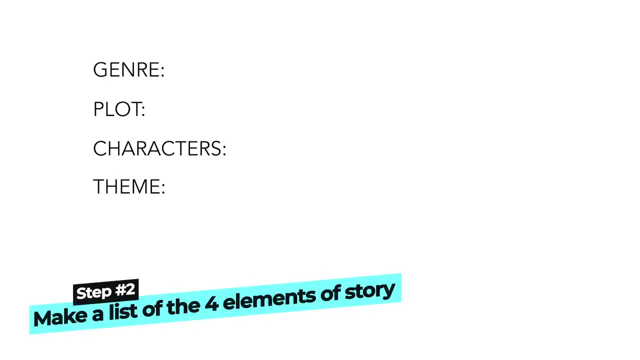 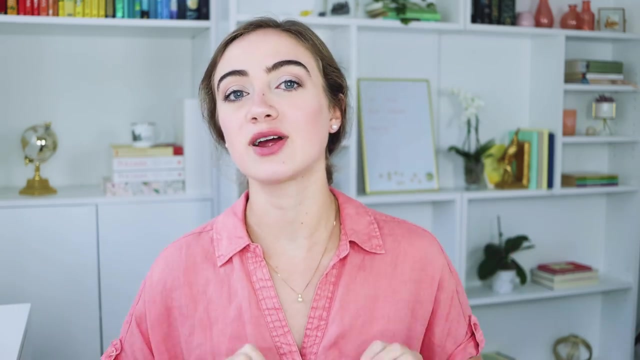 Okay, Once you have that list of stories, we're going to make another list of the four elements of story: Genre, plot, characters and theme. Choose one story for each of those categories and ask yourself: what is my favorite aspect of this story? Do I love the characters, the genre, the plot? 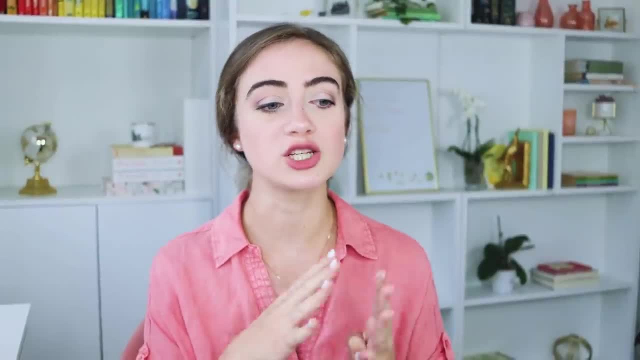 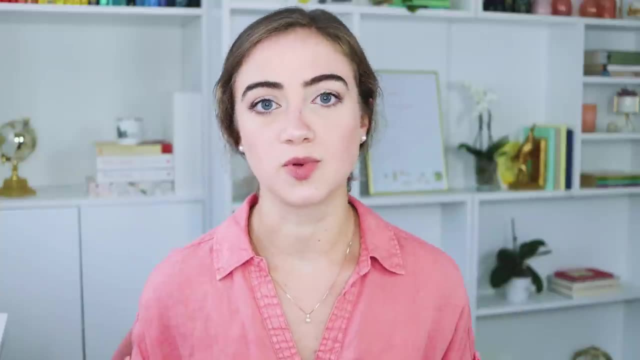 the theme And maybe you love all of those things about it. but try to choose what is the thing that stands out the most to me about this story that I'm like: oh, I love the plot, Oh, I love those characters and their relationships with each other. So 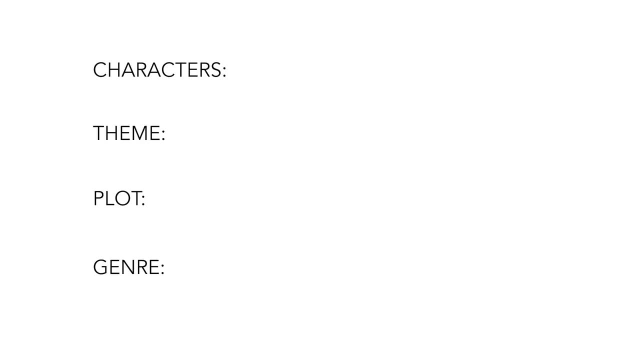 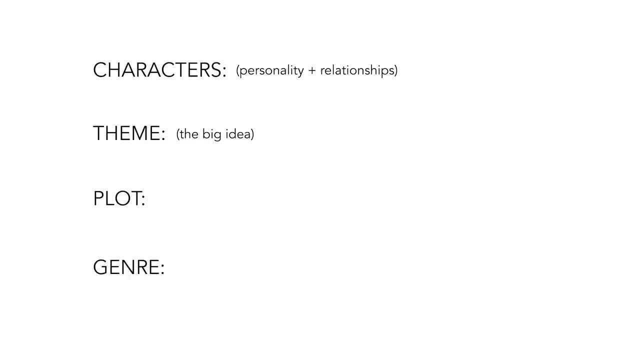 I'm talking about the big idea, the overarching message behind what the characters learn in their transformative journey. And when I say plot, I'm talking about the irresistible premise, the hook, the setup for all of the external events. And when I say genre, I'm talking about setting. 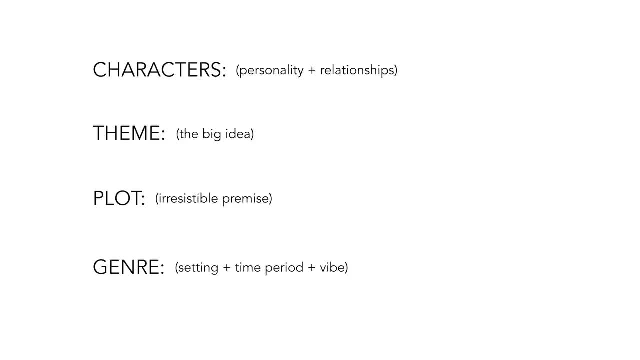 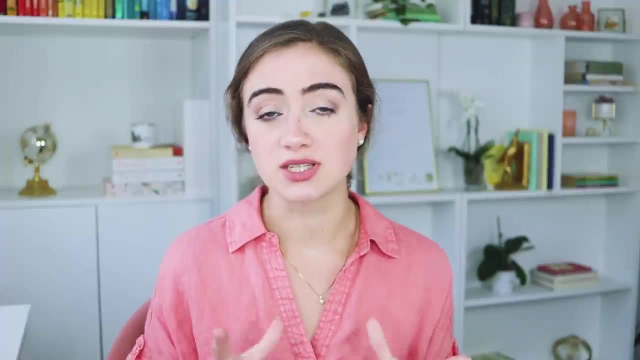 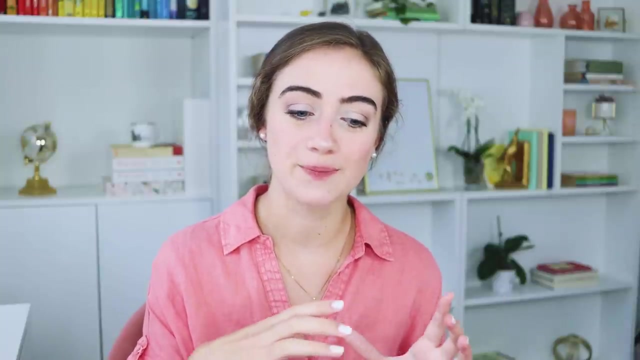 time period and the general vibe of the story. If you're writing a short story, not something as long as a novel or a series or something like that, you can do this exercise. Just choose your four favorite scenes instead of stories. So you're looking more at a smaller scope. You're looking at 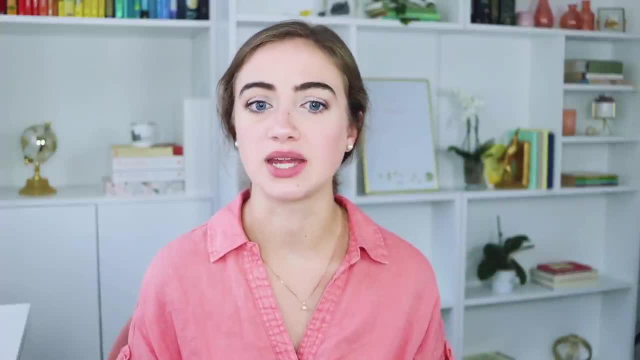 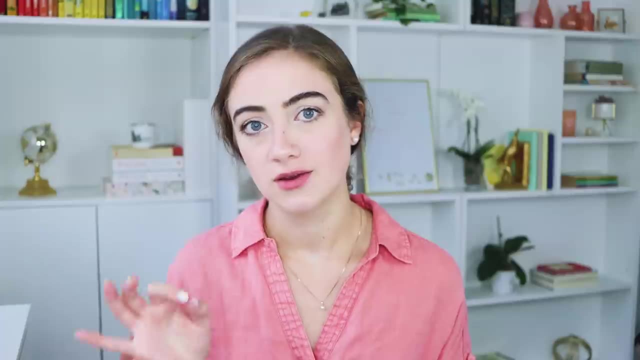 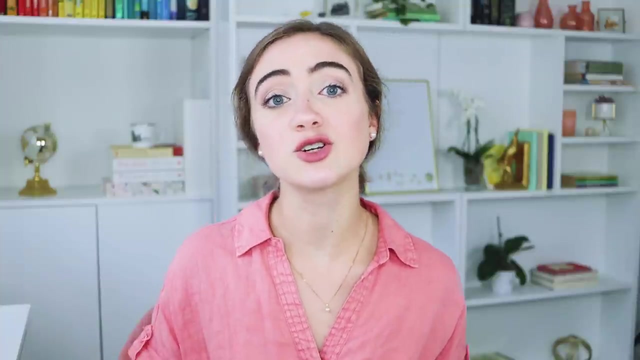 a single event or a day or something happening in a short period of time. So your four favorite scenes that you have recently watched or read. what did you love about them? Figure it out. Then go to your list of the four story elements: genre, plot, characters and theme. Choose what goes where. 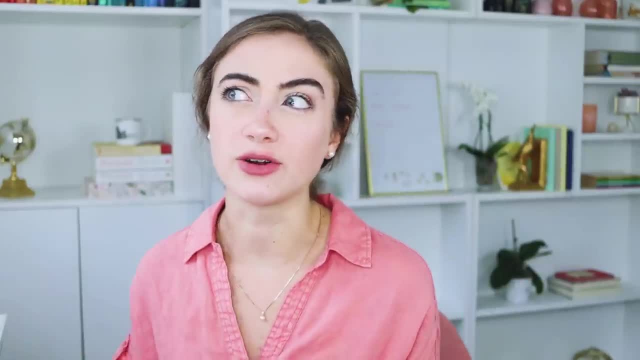 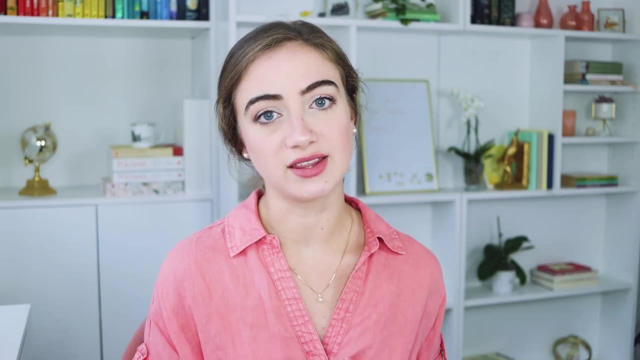 But wait, Abbey, Isn't this like just making a retelling of a story that already exists? Not quite, See. with most retellings, there are only two things that change: We're taking the same plot, We're taking the same characters, We're taking their relationship, their internal conflict. 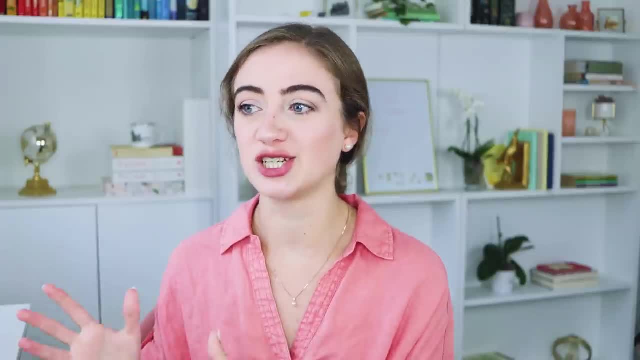 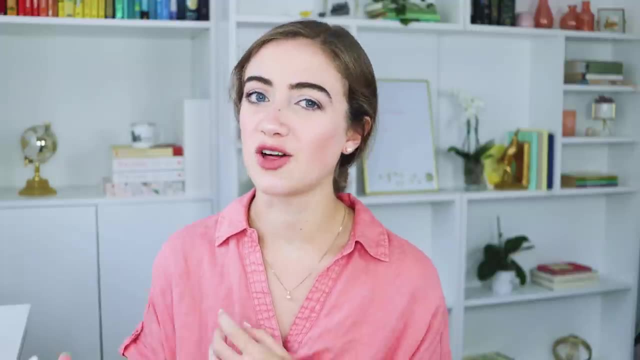 the theme, We're taking basically everything about it and we're just changing the genre or the time period. That's literally the only thing that happens with a retelling. usually, A lot of times, an author will add their own flair to the story and maybe add some subplots or something like that. 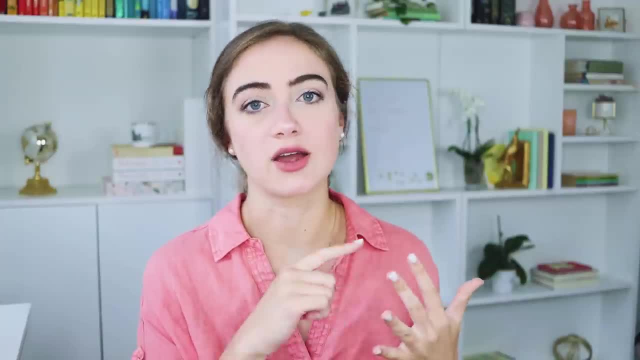 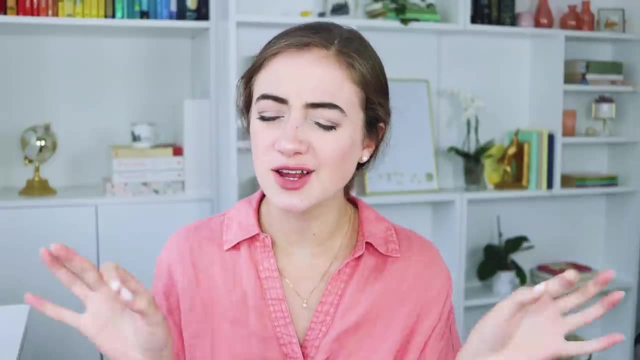 but they generally take the same story, the same plot, characters and theme and they just dress it in a different setting, a different tone, a different time period. That's not really what we're doing here. I'm not telling you to write retellings of stories. I'm 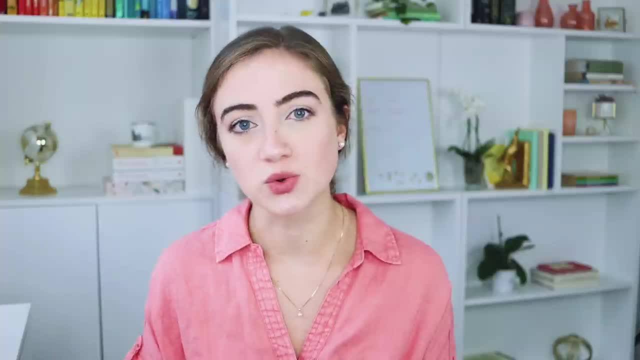 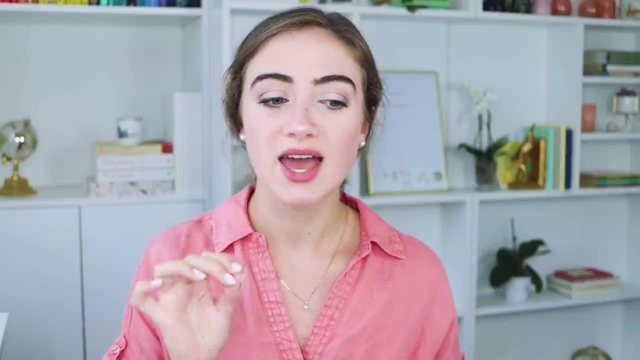 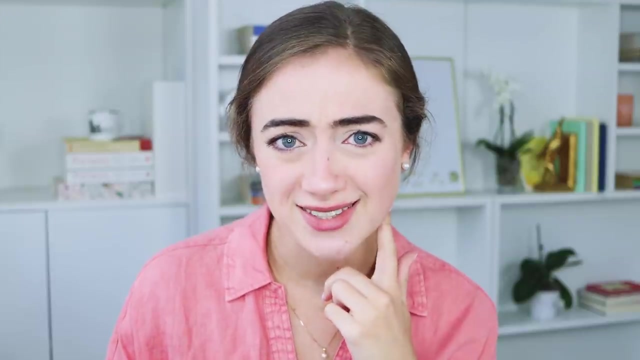 telling you to find the things about your favorite stories that get you really excited and inspired, and extract those small elements from those stories and rearrange them to create your own unique thing. Do writers, Do writers really do this? Yeah, actually they do. Here are some examples: The Twilight series is inspired by a bunch of 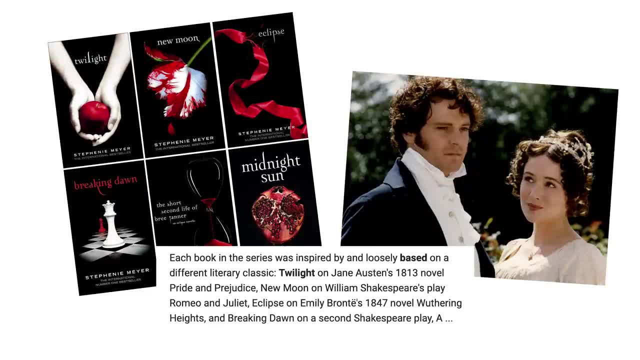 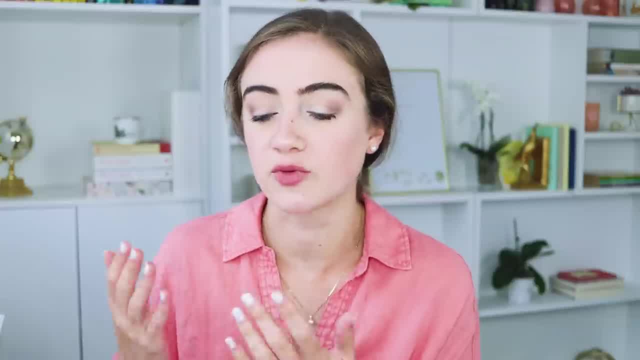 classics, including Pride and Prejudice. While you're reading Twilight, are you thinking, wow, this is like literally Pride and Prejudice. I can't believe she just stole Pride and Prejudice. I feel like I'm reading Pride and Prejudice. No, you don't think that at. 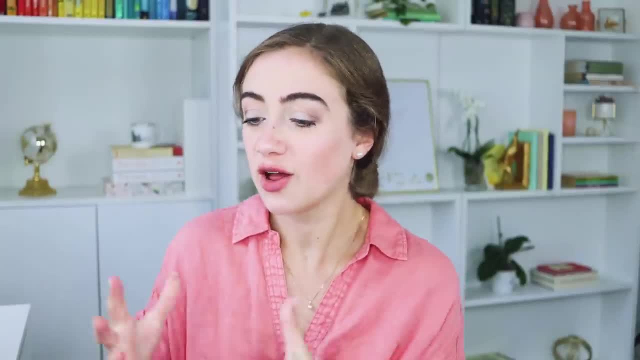 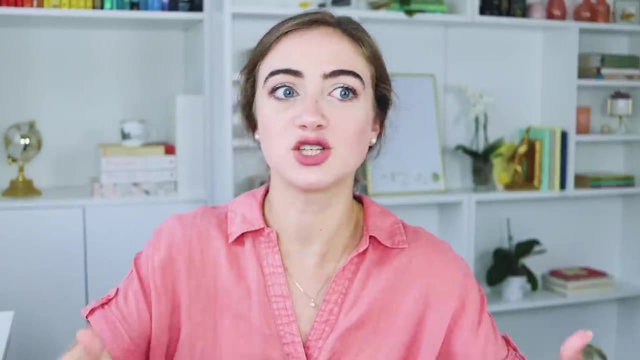 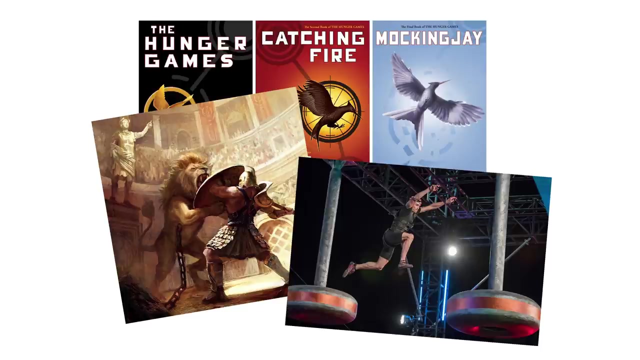 all It's unrecognizable because she changed the whole genre and made it her own thing. And how many do you think are inspired by Twilight now? And so it goes on. Some other examples: The Hunger Games was inspired by gladiators, and televised challenges- You've Got Mail- was inspired by. 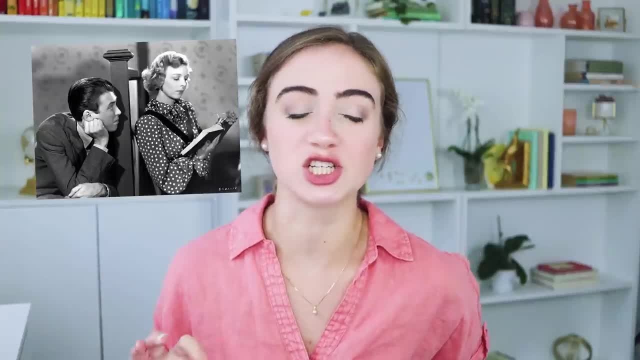 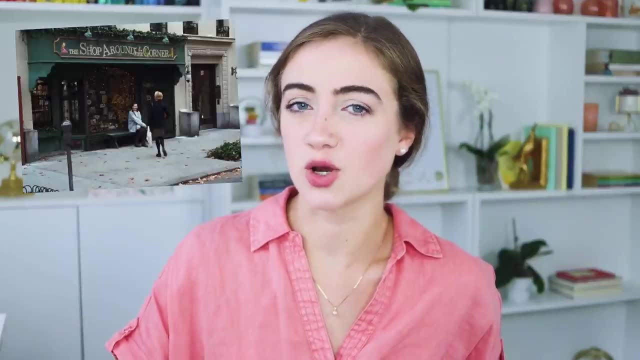 the old film The Shop Around the Corner, which is such a cute movie, And I didn't even know that until I saw that older movie and I'm like, oh my gosh, Good shout out, though, making Meg Ryan's character own a store called The Shop Around the Corner. See, that's a respectful nod to stealing. 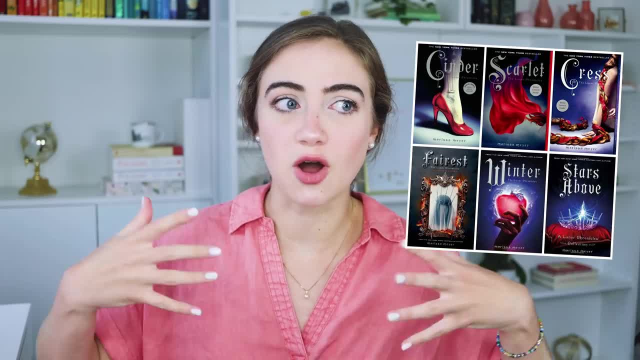 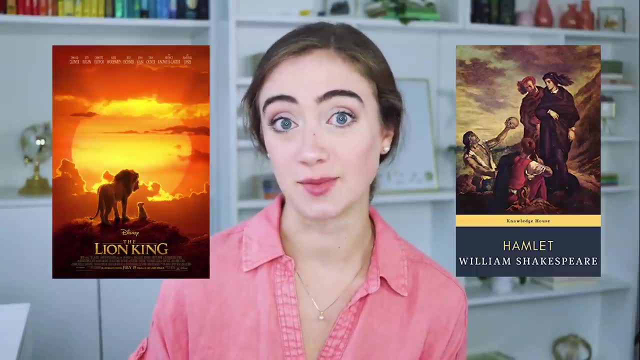 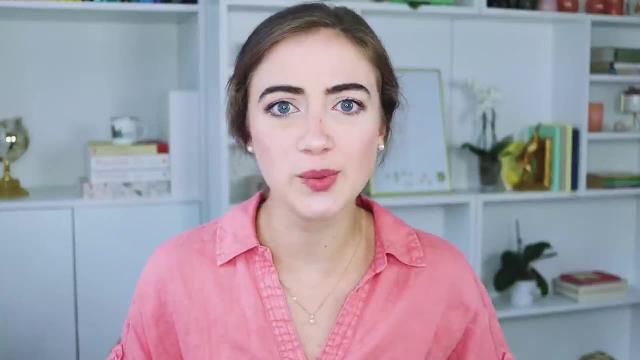 stealing from another artist. The Lunar Chronicles are fairy tale retellings Meet science fiction, And The Lion King is basically Hamlet. In other words, everything has been done before, and every writer steals from every other writer. So what are you waiting for? 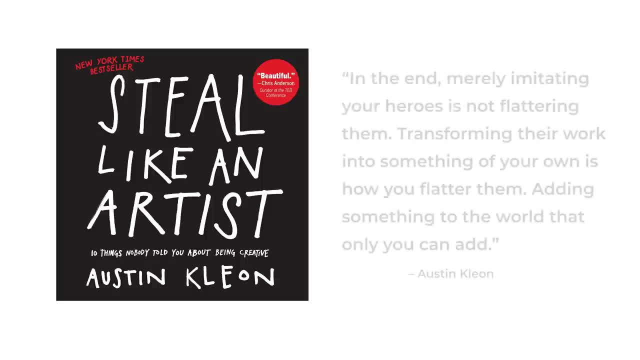 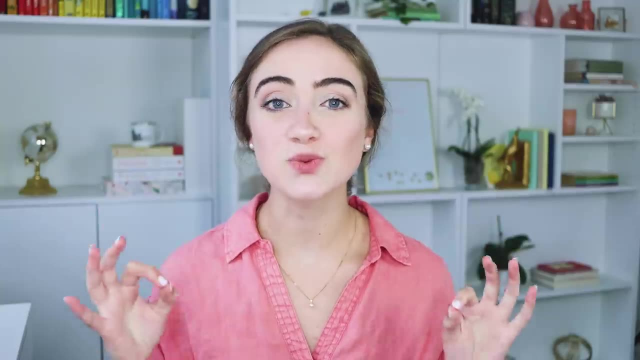 In his book Steal Like an Artist, Austin Kleon says: in the end, merely imitating your heroes is not flattering them. Transforming their work into something of your own is how you flatter them, Adding something to the world that only you can add. That's what I'm. 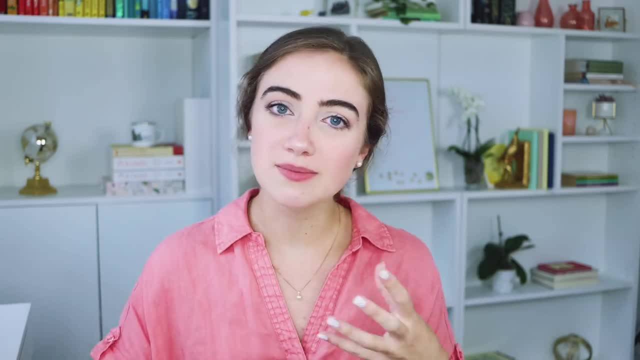 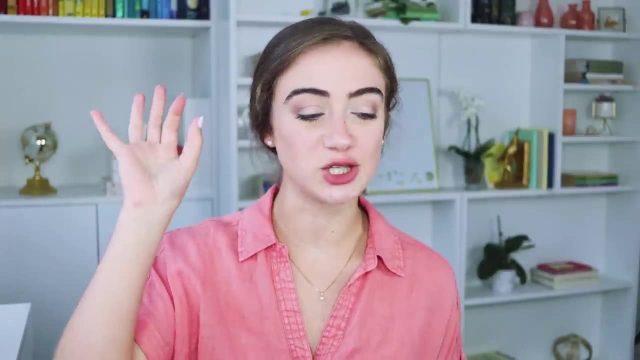 talking about, with the unique arrangement, your own remix of the things you love about your favorite stories. So make a master list of your favorite stories that get you the most excited and creatively inspired, And then make that list of the four story elements: characters, genre. 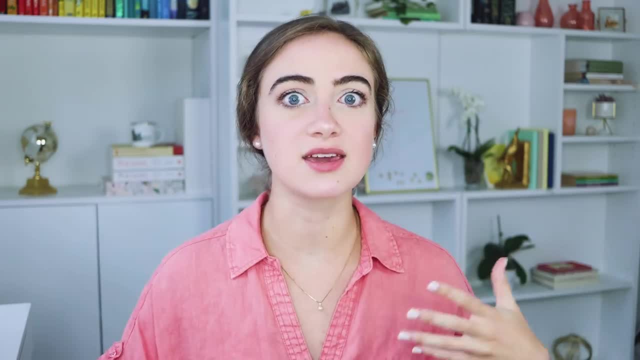 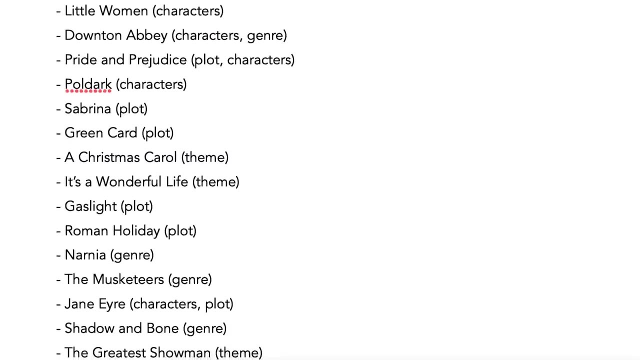 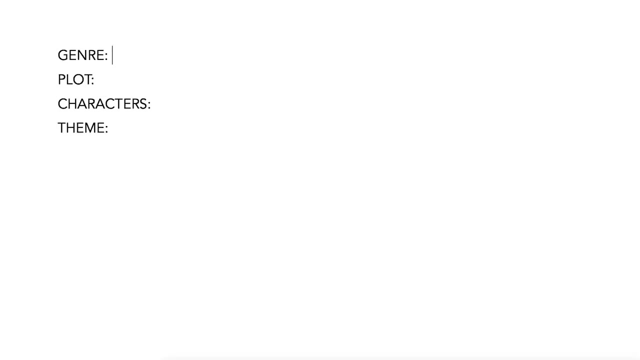 plot and theme and start mixing things up. And if you're still like, how do I do this Exactly, Let me show you an example. So I've started making a master list of some of my favorite stories. Genre: Um, oh gosh, there's so many to choose from, So many I love. I'm going 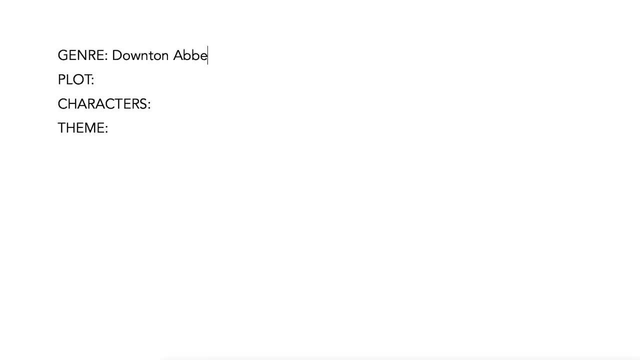 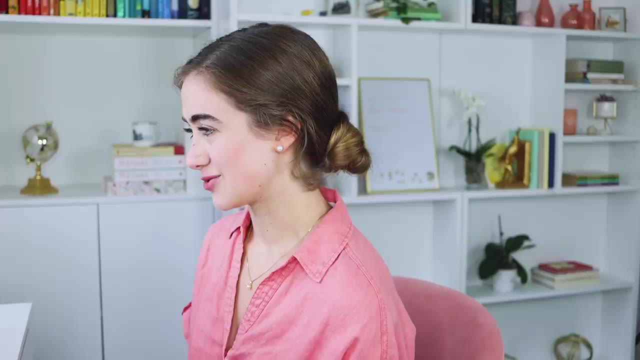 to choose this genre of Downton Abbey. So like early 1900s posh English society Plot, Let's take something I've seen recently. I'm going to take the plot of Sabrina, Such a cute movie, Love. 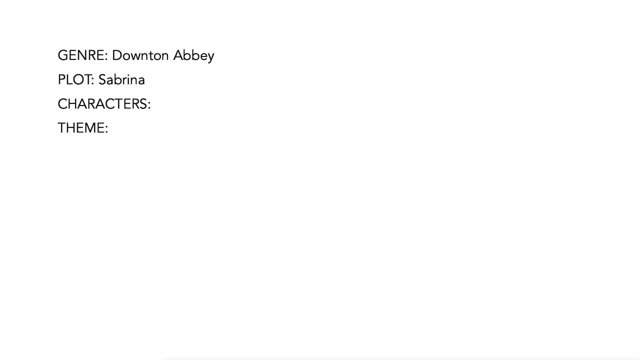 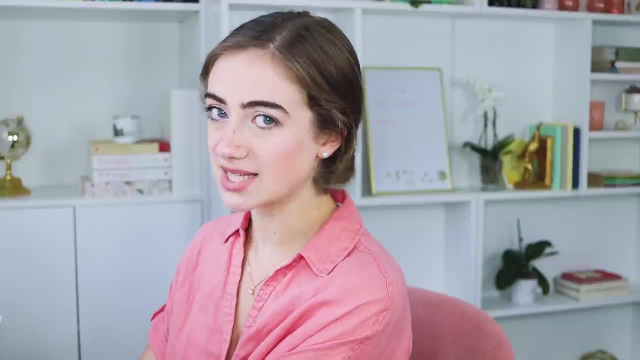 love that premise And the characters. Let's take the characters from one of my favorites, Poldark. If you guys haven't seen Poldark, you are missing out. Okay, For the theme, you're going to want to take something that works with these different 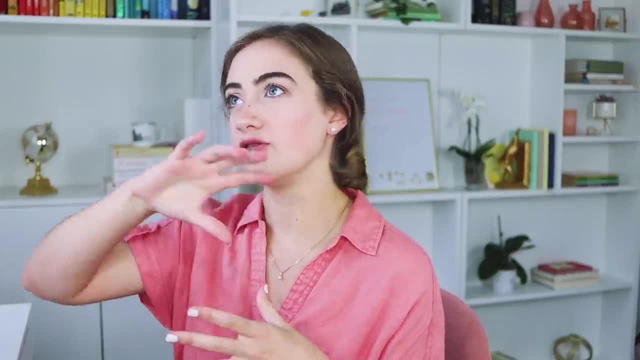 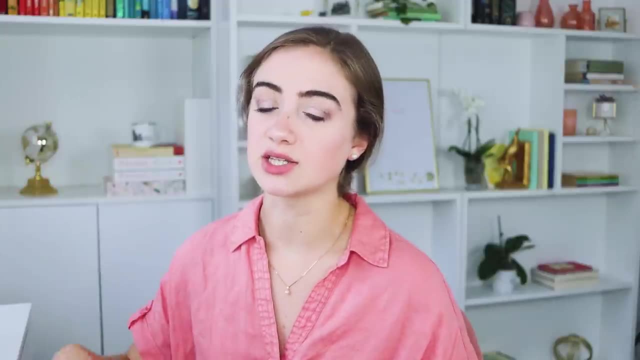 elements, especially with the plot. So, as we always talk about on this channel, the external conflict and the internal conflict, and the journey that your character goes on leads them to their aha moment, leads them to the big idea. So the big idea is kind of the thing. 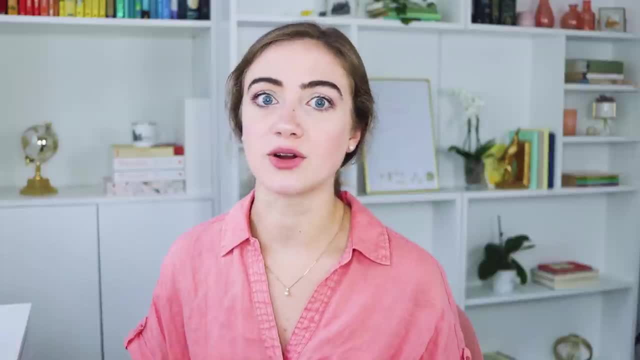 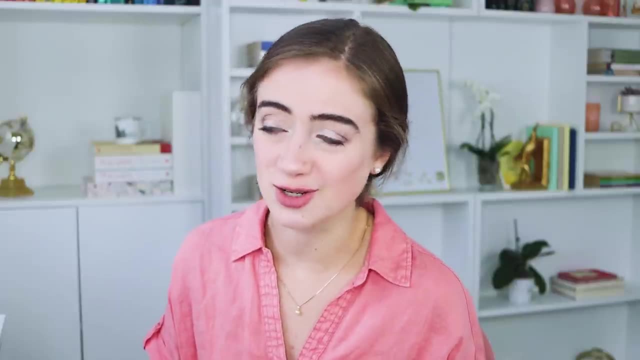 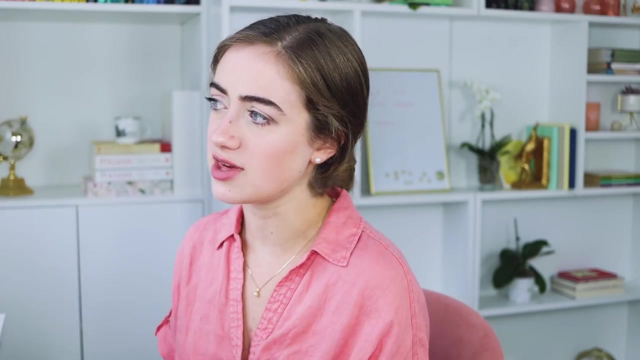 that you have to come up with first And reverse engineer how they're going to arrive at this big idea. So you're going to want to pick a theme that compliments the plot and the characters. You don't want something way, way off, Okay. So kind of just use your common sense here. Pick a theme from your list here. 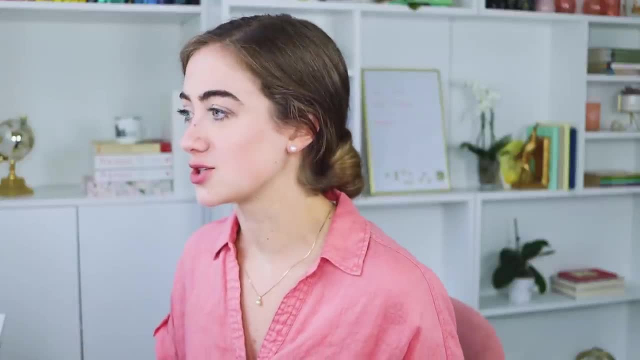 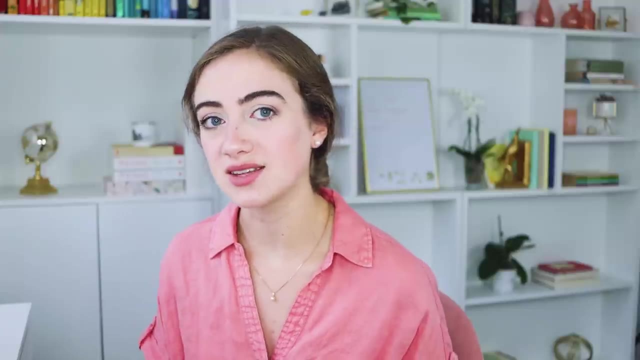 that matches, or could match, with your characters. It can even cross over a little bit, because a lot of themes repeat across different stories And it's the way that the story presents that theme that makes it unique. So I'm going to take the same theme as in Sabrina. 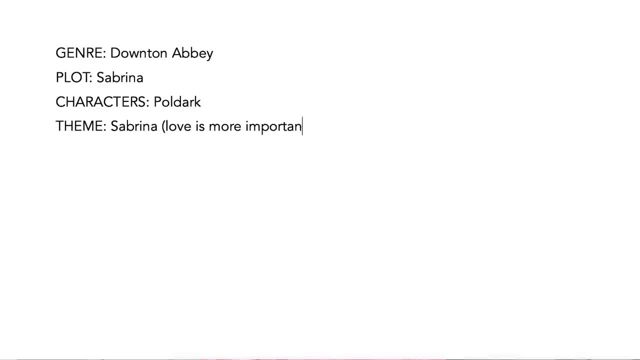 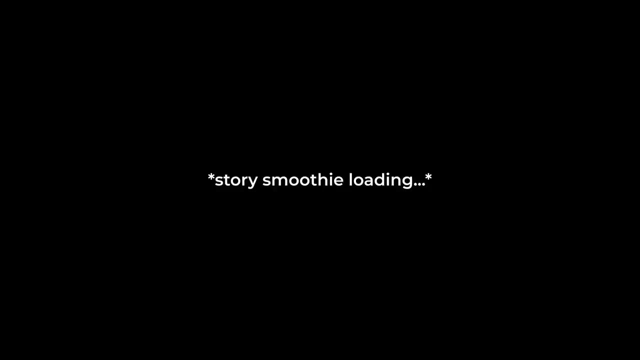 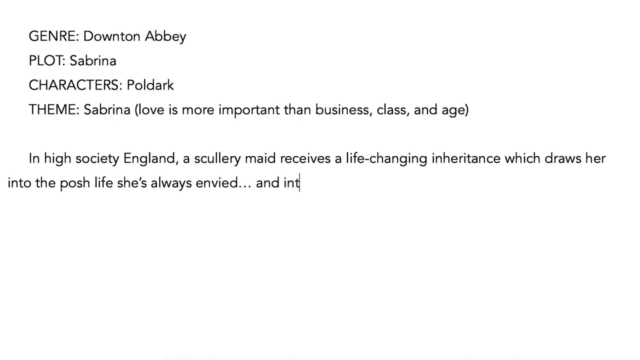 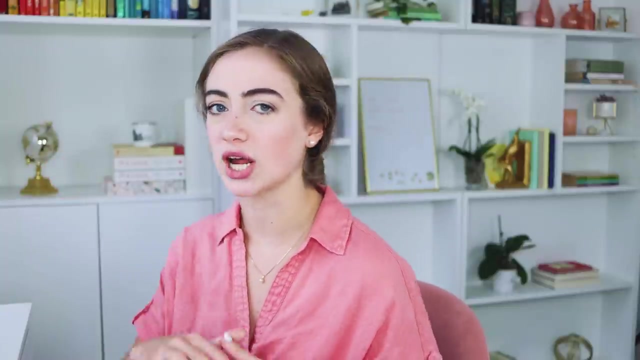 which is kind of that: love is the most important thing. It's more important than business and class division and age and all of that. Okay. So now we have a good concept, a concept that I can get excited about, because I love Downton Abbey and Sabrina and Poldark. I love all these stories. They're great And I can 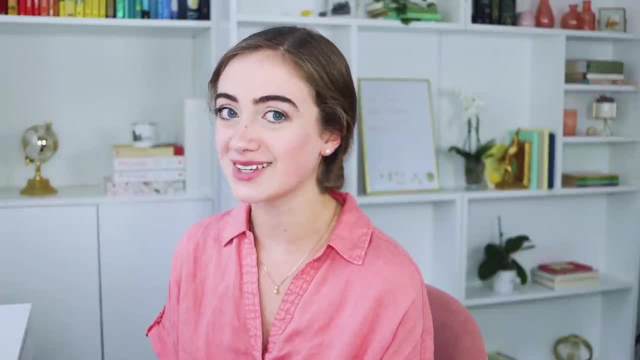 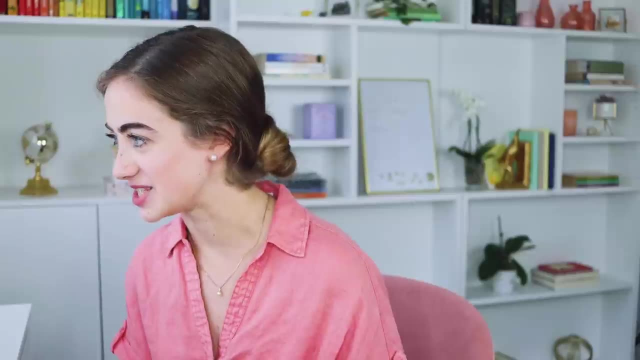 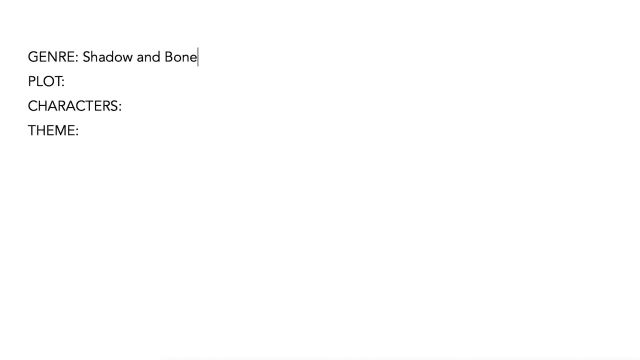 take these different elements and remix them to be something unique. Let's do another one, Something kind of different, darker and more mysterious. Genre, genre, genre- What do I want for my genre? I just recently read the Shadow and Bone trilogy. I really liked that genre. 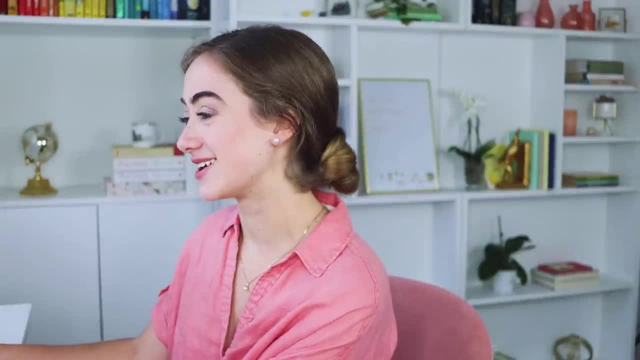 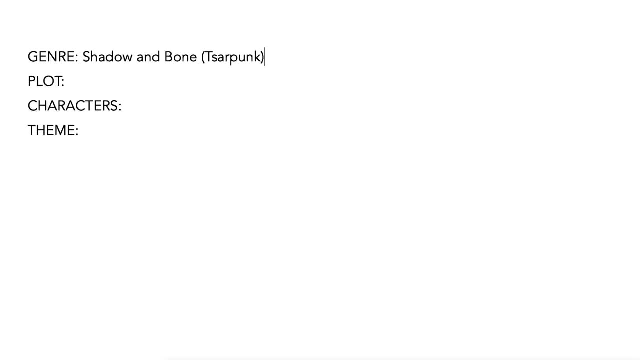 I didn't think I was going to like that genre, but I really like it. Okay, So we'll go with that. We'll go with, like a World War I fantasy, Tsar, punk And for the plot, gosh. y'all know I love. 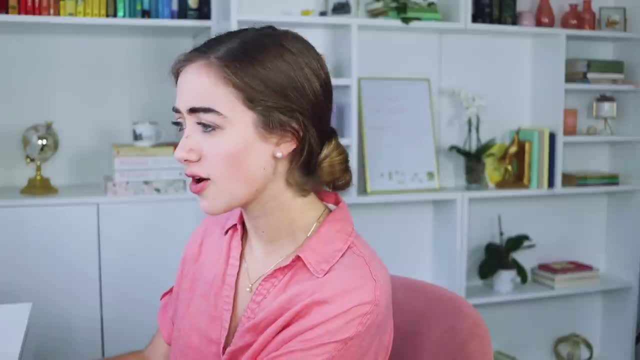 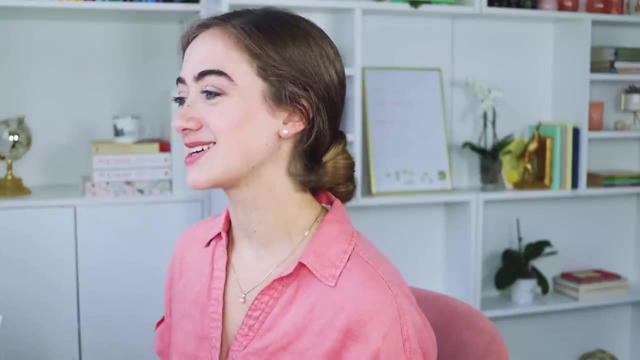 Tangled, Let's use the plot of Tangled And for the characters, let's use the characters from Jane Eyre, because it's an old favorite and it still gets me inspired. Now theme: I want something that is not too different from Tangled. 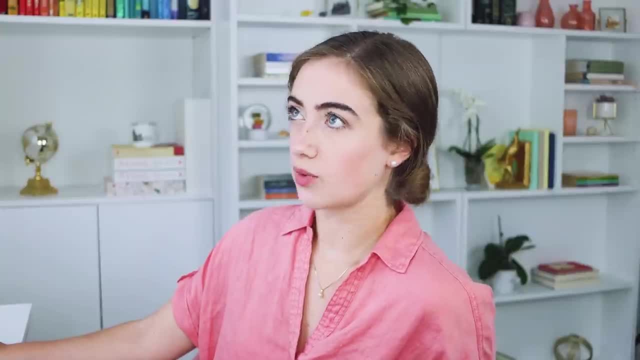 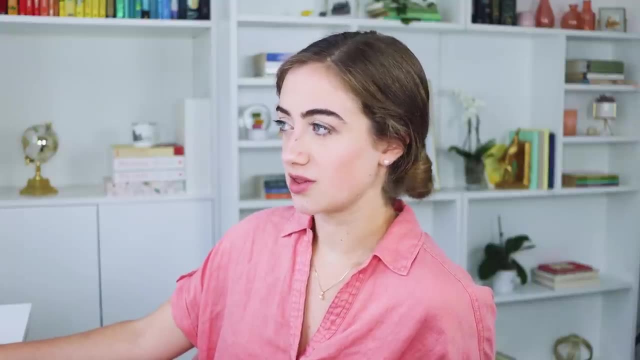 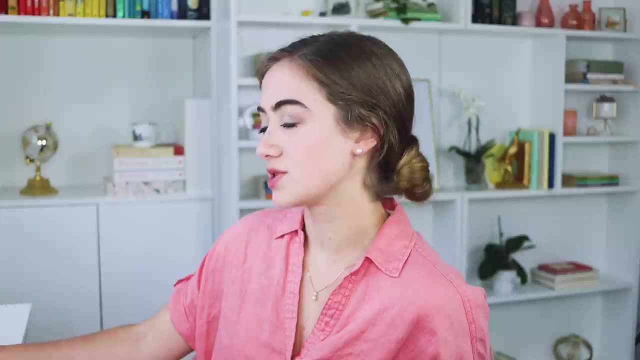 so this one's going to be like more dark and mysterious, So I don't want it to be like too much of a happy Disney princess theme. Tangled does deal with like emotional manipulation themes, So I'm going to take the theme of Gaslight, which is one of my favorite old films, Also missing out. 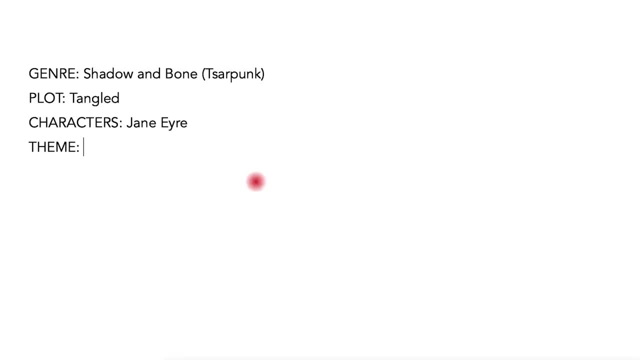 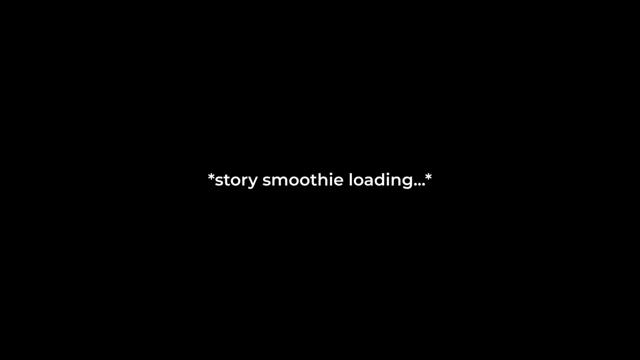 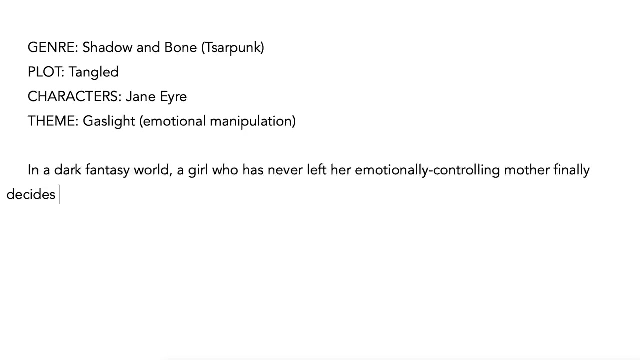 if you haven't seen that Ingrid Bergman, So good Gaslight, because it's going to cover some themes of emotional manipulation. Let's do one more, Something kind of fun and adventurous Genre. What do we want for our genre? Maybe something totally different: Sci-fi, Star Wars. 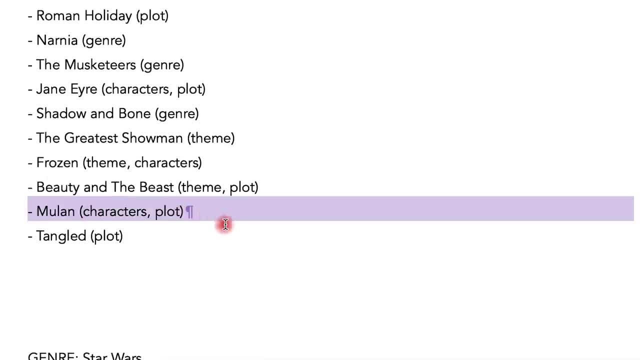 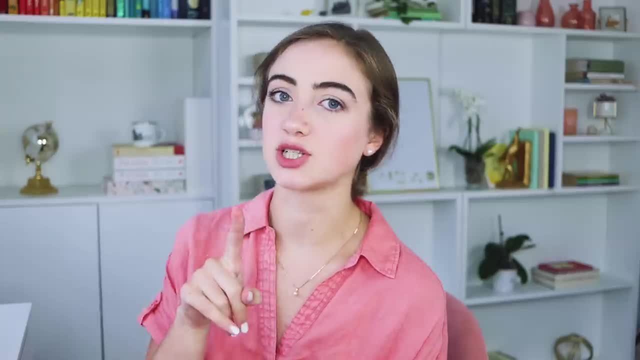 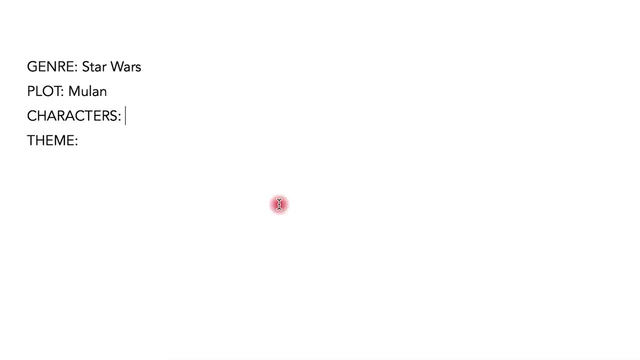 And plot, Plot, plot, plot, plot. Let's take another Disney movie. Those old movies have good plots. Let's do the plot of Mulan, The original film, that is The new one- Fucked Characters. Oh, you guys are wondering why I haven't talked about Pride and Prejudice yet. 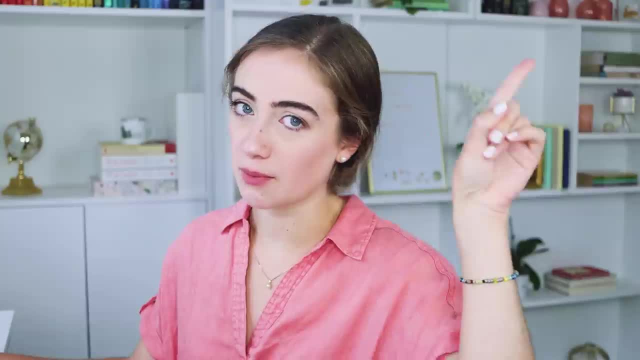 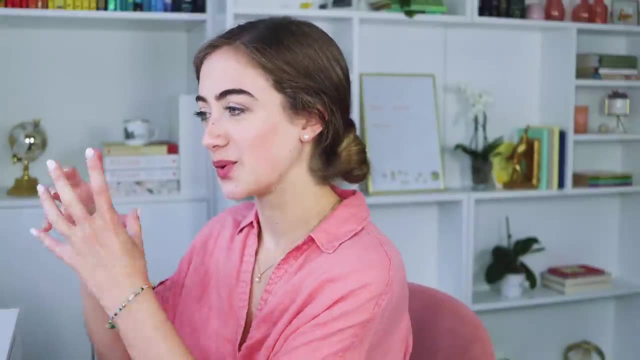 Let's do Pride and Prejudice for the characters. You know I love these characters more than most people in real life. And theme: Okay, we want this to be kind of inspirational, So let's remix within the remix. I'm going to take a combination here of the theme from Mulan and the theme from Pride. 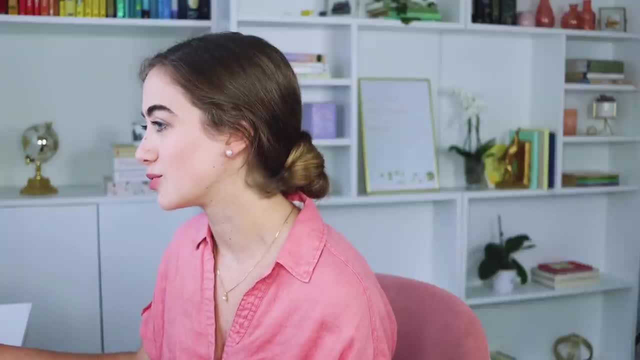 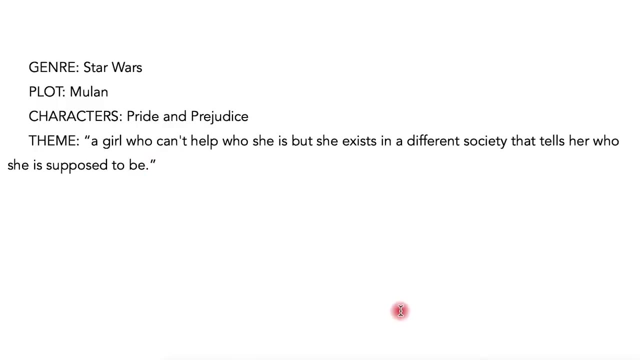 and Prejudice, because they're kind of similar. I was looking up the theme of Mulan and this is the first thing that came up. It's something that the co-director said: a girl who can't help who she is, but she exists in a different society that tells her who she's supposed to be. 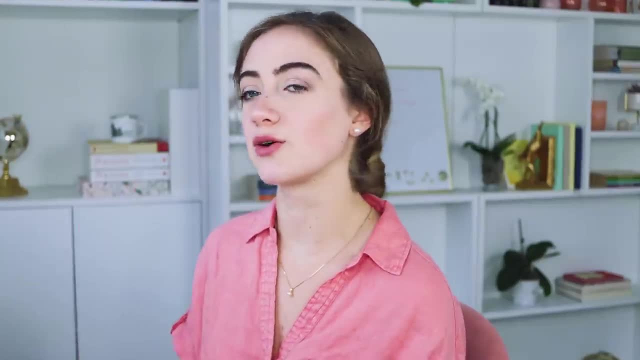 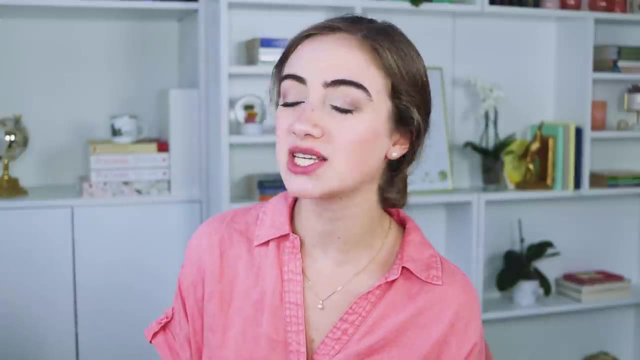 That kind of sounds like Lizzie Bennet, doesn't it? I mean, that's going to be the broad overarching theme. A lot of stories have done it. This make believe story is going to do it, but it's going to be a space adventure like Star Wars. 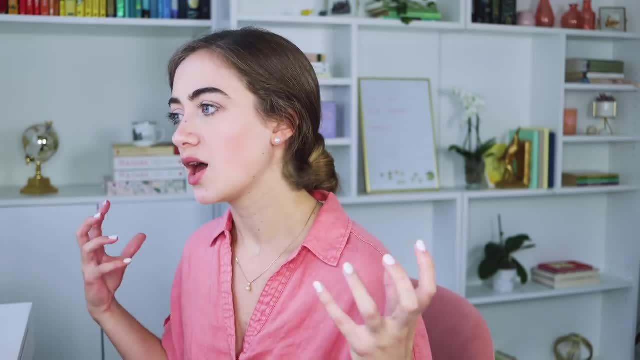 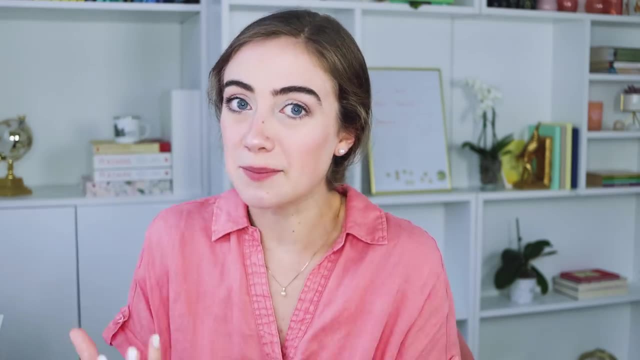 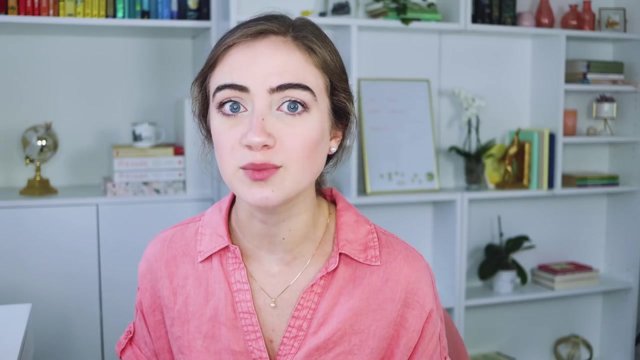 Literally just came up with that in two minutes and I know it needs more detail, but this is something that you can get excited about, because you can take stories that matter to you personally, that you have prior emotional connections with. Okay, Like I talked about in the beginning, that's why writing prompts don't work. 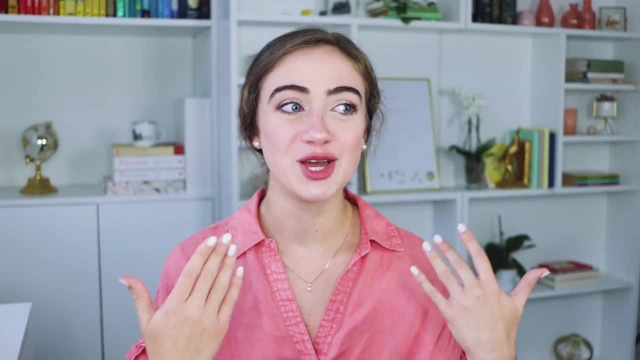 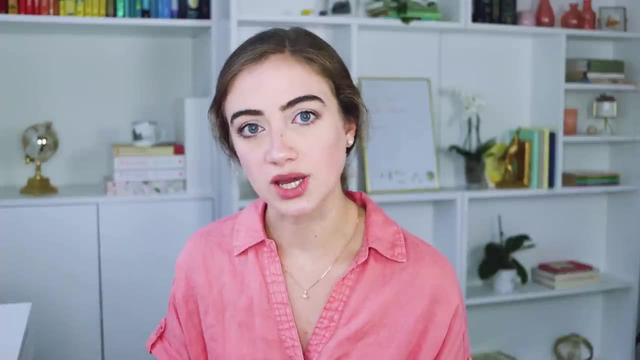 because you don't care. They're out of context. Who cares? You don't. How will your readers care? Your excitement, your passion for these elements of story will come through your writing. That is going to be what shines through your writing, because you have passion for this.